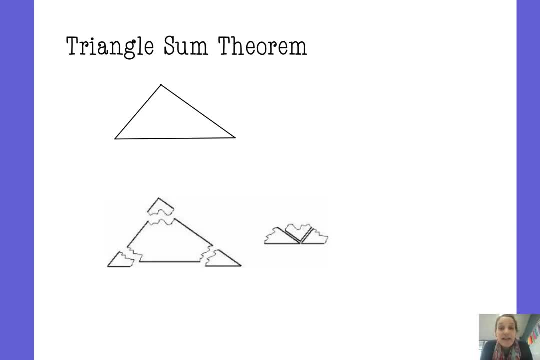 The next thing we're going to learn about is called the triangle sum theorem. So let's say we have this triangle. It has three angles. Here's an angle, here's an angle, here's an angle. So maybe we'll color them. So it has three angles. 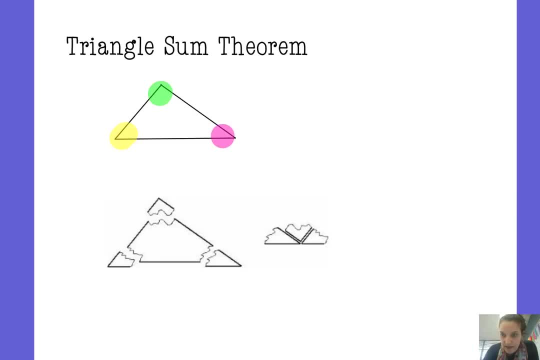 So if you had a triangle, you can actually cut one out of a piece of paper and do this with me. If you ripped off the corners, just like you can see in this picture, if you went and ripped off the corner angles and removed them from the triangle and then went and stuck them all together and had all their vertices. 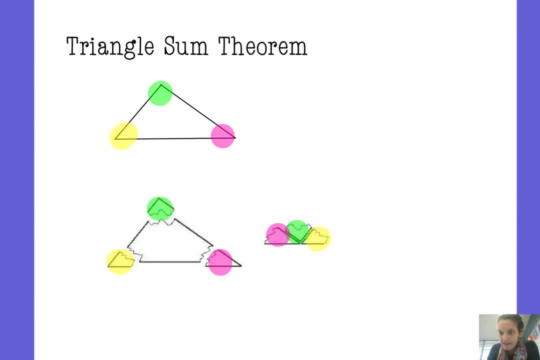 touching, you would notice that when you stick those three angles together, this is a straight line. I just created a straight angle. How many degrees are there in a straight angle? 180 degrees. So what this proves is if you add the measures of these three angles- the pink angle, the yellow angle and the green angle. if you add the three, 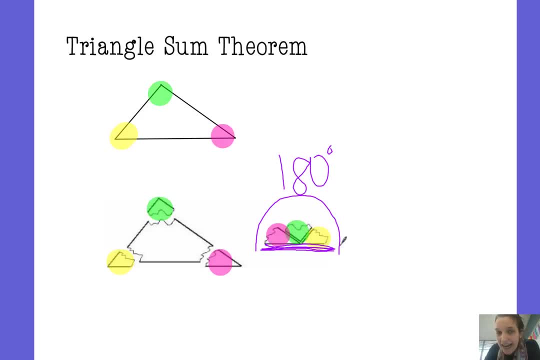 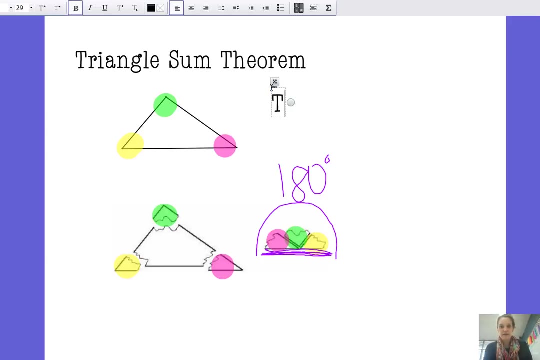 of a triangle. together, they will always add up to 180 degrees. so the sum of the angles of a triangle will always be 180 degrees. so if the sum of the three angles of every triangle will always be 180 degrees, that is what the triangle sum theorem says. if you add up all the angles, they will always be 180 degrees. 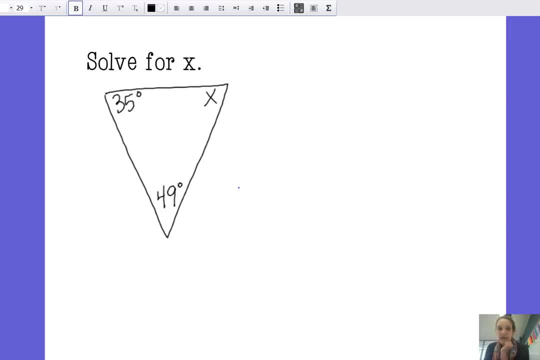 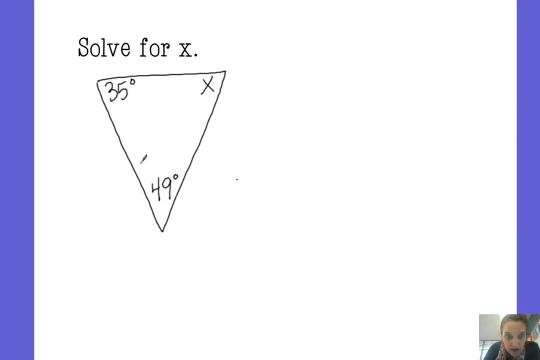 so if we look at this example, I know to my angles and I'm trying to find the third angle, X. well, I know by the triangle sum theorem that if I add those three angles together they should add up to 180. so I should be able to say 35. 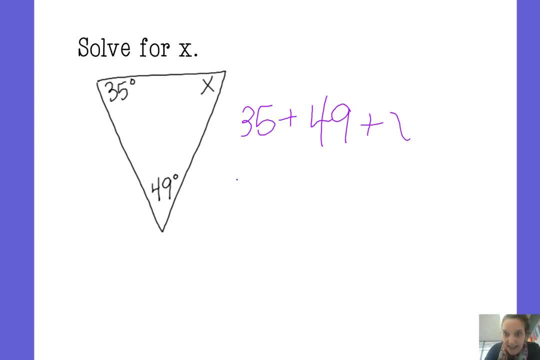 plus 49 plus X, adding those three angles together- angle plus angle plus angle- should add up to 180. so I can come by my terms: 35 plus 49 is 84, and then I can subtract 84 from both sides and that should give me X is 96. so 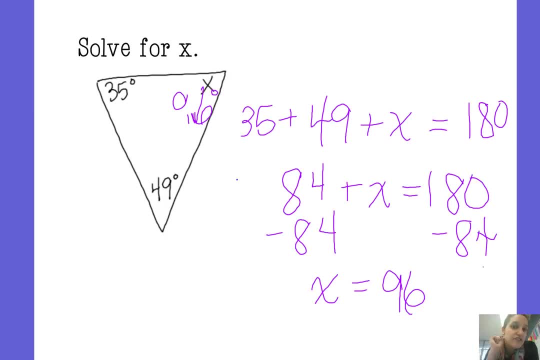 if X is 96 degrees and I need to classify this triangle based on its angle measures, since 96 boy 90. so mercies. since 96 is an obtuse angle, it's bigger than 90 degrees. this would be an obtuse triangle. here's another. 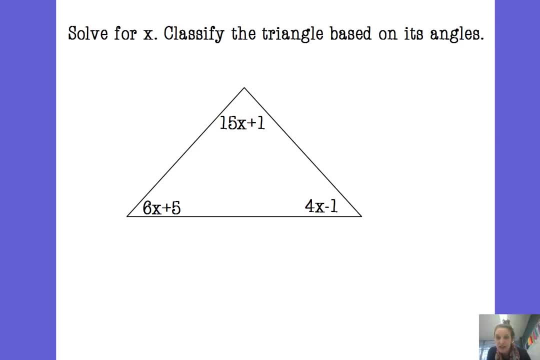 example, solve for X. classify the triangle based on its angles. so I have my three angles. I have expressions to represent my three angles. I know by the triangle sum theorem, if I add up these three angles they should always add up to 180 degrees, so I can say 6x plus 5. come on touchscreen. this is your time to. 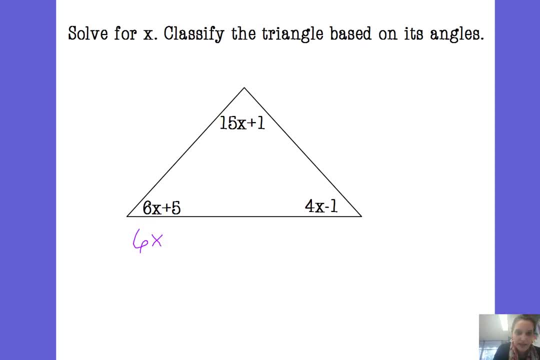 shine. don't be mean 6x plus 5 plus 15 X plus 1 plus 4 X minus 1. if I add up those three angles they should add up to 180 in every triangle I can add up all the angles. set them equal to 180. so I'm going to add my light terms: 6 X, 15 X and 4 X. 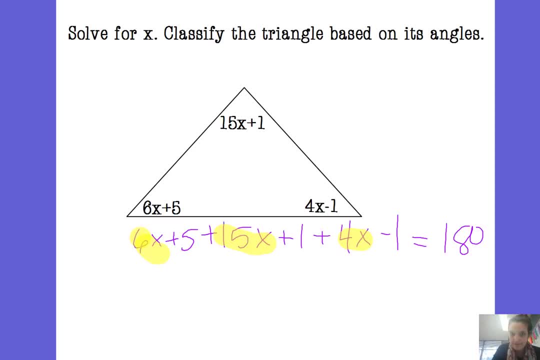 gives me 25 X, and then I can add all my whole numbers: 5 plus 1 is 6,, 6 minus 1 is 5, then I'm going to subtract 5 from both sides- 25x equals 165,- oh no, not 15,, sorry- minus 5, 175, and divide. 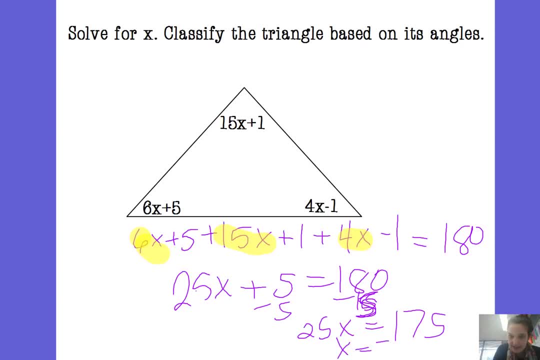 by 25 and you get x is 7.. So now what I can go do is go plug 7 back in for x. 4 times, 7 is 28,. minus 1 is 27 degrees. 6 times 7 is 42,, 42 plus 5 is 47 degrees, and then 15 times.